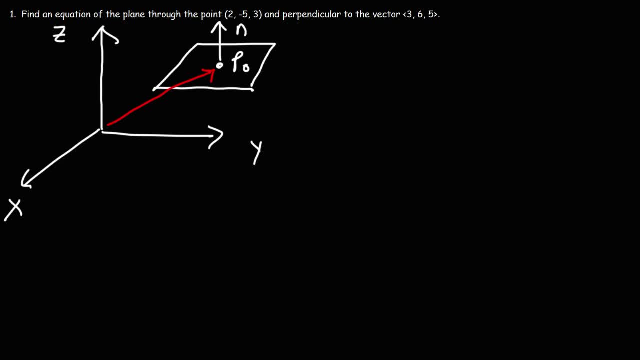 the origin going to p0. So we're going to call this r sub 0. And we're going to have another point on this plane which we'll call p, And so we're going to have a position vector that points towards that as well. 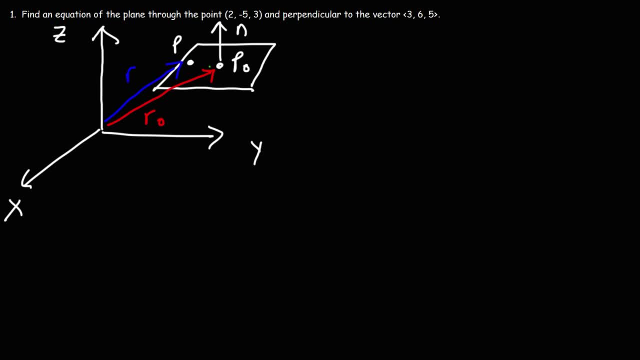 Which will be r, Now going from p0 to p. this is going to be another vector, which we'll call r minus r0.. r minus r0, that's going to be equal to this vector, which goes from p0 to p. 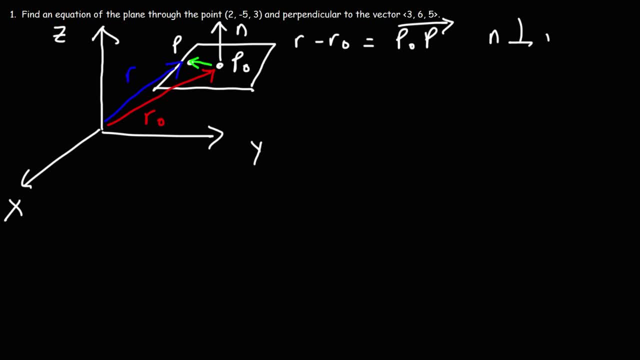 Now keep in mind n is perpendicular to that vector. Because it's perpendicular, the dot product between the normal vector and the vector r minus r0, that's going to equal 0. Because those two vectors are orthogonal to each other. Now the vector n, the normal vector, will be represented. 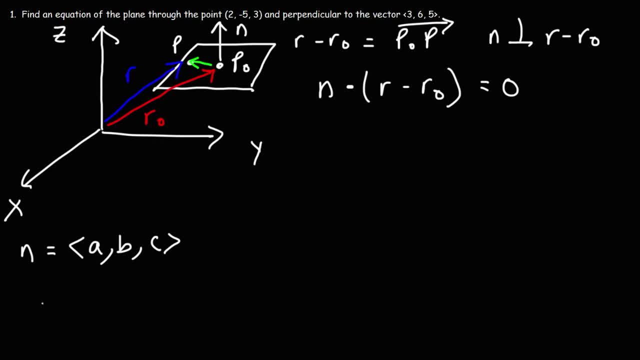 by these values: a comma, b comma, c, r is going to equal xyz. This is based on point p and r0 is going to equal the vector, based on p zero, which will have the points. I mean the values x zero, y zero, z zero. 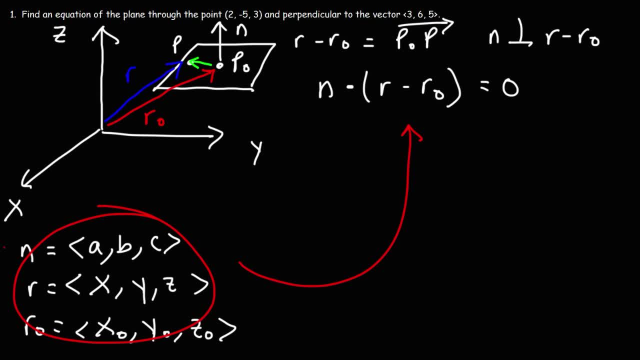 Now let's take these values and plug it into that formula. So n is going to be a comma b, comma c, And then r minus r, zero. I'm going to run out of space, So let me put this somewhere else. So here's n, And then we have the dot product of that with. 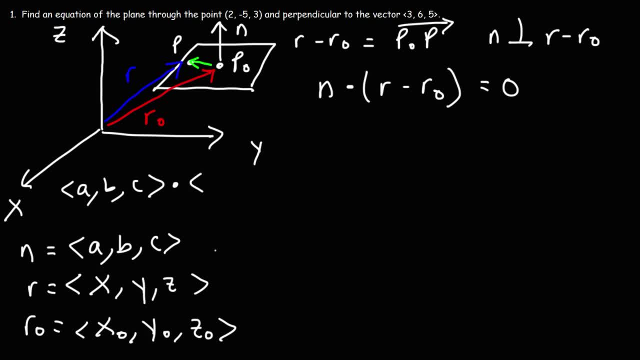 r minus r zero. So this is going to be x minus x zero, And then comma y minus y zero, And then comma z minus z zero. So, using the dot product formula, we're going to have a a times x minus x zero, And then b plus b times y minus y zero. 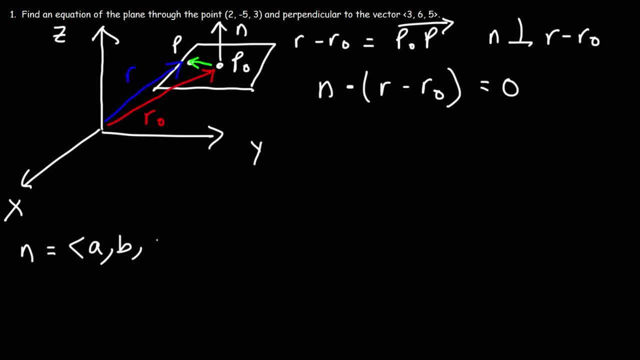 will be represented by these values: a comma, b, comma c. r is going to equal xyz, which is based on point p, and r0 is based on p0, which will have the points. I mean the values x0, y0, z0. 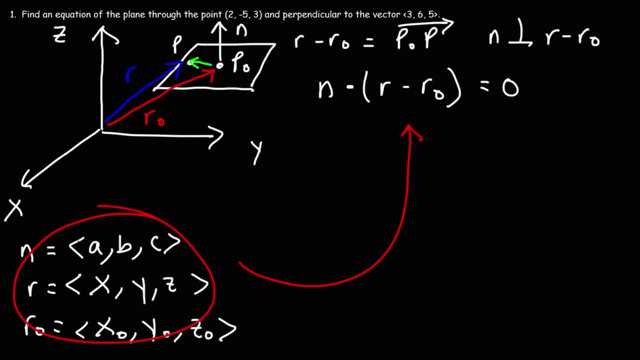 Now let's take these values and plug it into that formula. So n is going to be a comma b, comma c, and then r0 is going to be a comma b, comma c, And then r0 is going to be a comma b, comma c, And then r0 is going to be a comma b, comma c. 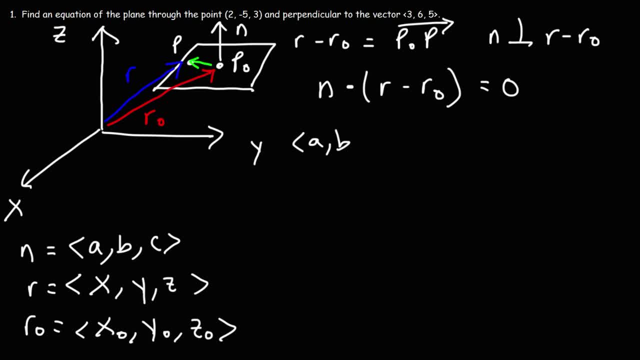 r minus r0,. I'm going to run out of space, so let me put this somewhere else. So here's n, and then we have the dot product of that with r minus r0.. So this is going to be x minus x0,. 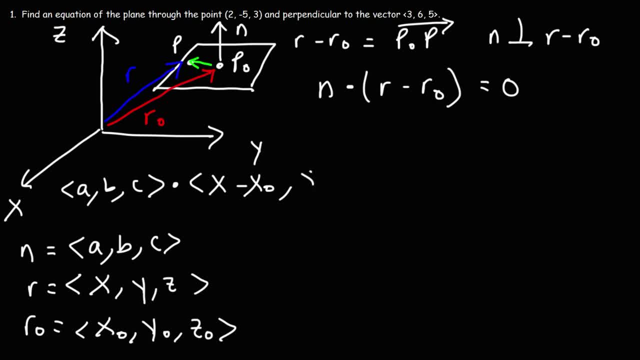 and then comma y minus y0, and then comma z minus z0.. So, using the dot product formula, we're going to have a times x minus x0, and then b plus b times y minus y0, and then plus c times z minus z0.. So all of this is going to equal 0. And this is the. 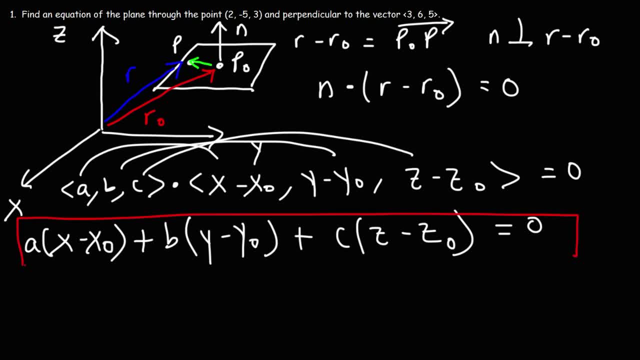 formula that we're going to use. that's going to help us to get the equation of the plane, given a point on a plane and the normal vector, So a, b and c, that's 3,, 6, and 5.. x0 is 2, y0 is negative. 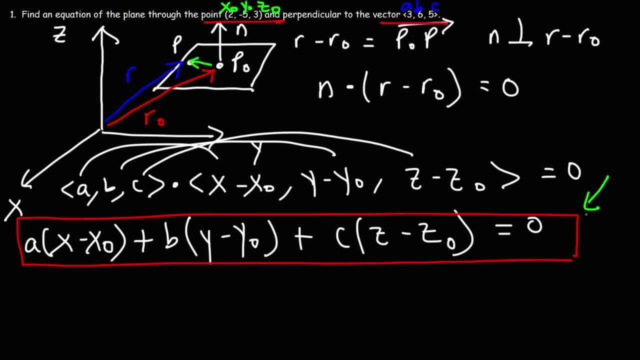 5, z0 is 3.. So we just got to plug that in into that formula. So let's replace a with 3,, x0 with 2, and then b is 6, and then we're going to replace y0 with negative 5.. And then c is 5,. 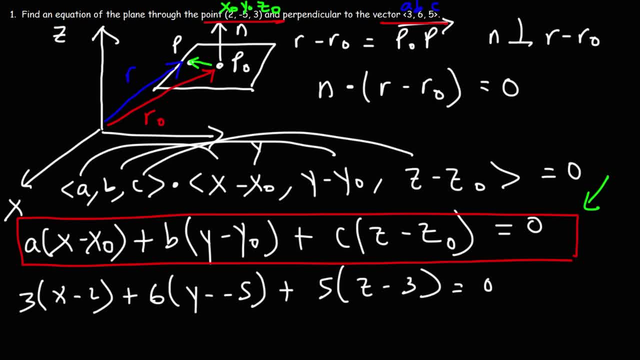 and z0 is 3.. So now we need to distribute. This is going to be 3x minus 6.. This becomes y plus 5 times 6.. That's going to be 6y plus 30, and then plus 5z minus 15,, which equals 0.. 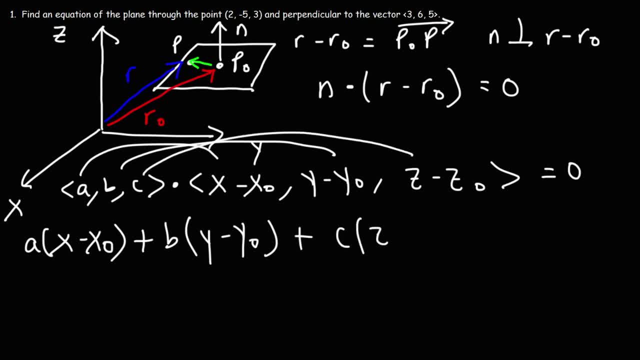 And then plus c times z, minus z, zero. So all of this is going to equal zero And this is the formula that we're going to use. that's going to help us to get the equation of the plane: given a point on a plane and the normal vector. 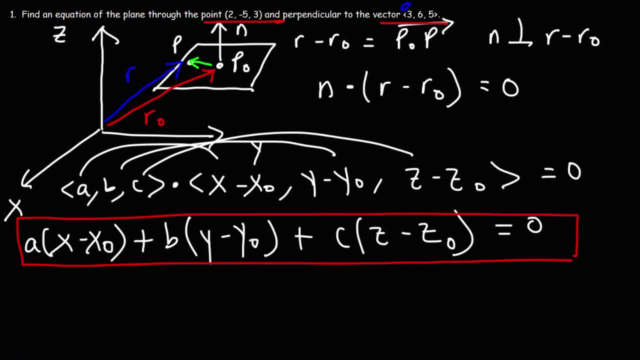 So a, b and c, that's three, six, and five x zero is two. y zero is negative, five z zero is three. So we just got to plug that in into that formula. So let's replace a with three, x zero with two, And then b is six, And then we're going. 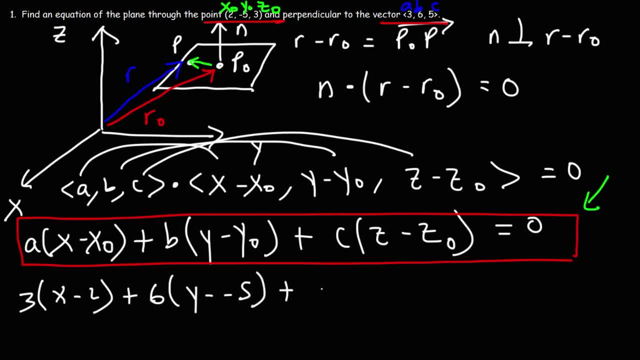 replace y zero with negative five, And then c is five And z zero is three. So now we need to distribute. this is going to be three x minus six. this becomes y plus five times six. that's going to be six y plus 30. And then plus five z minus 15,. 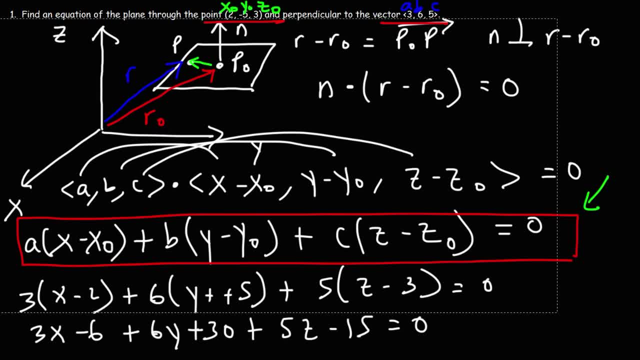 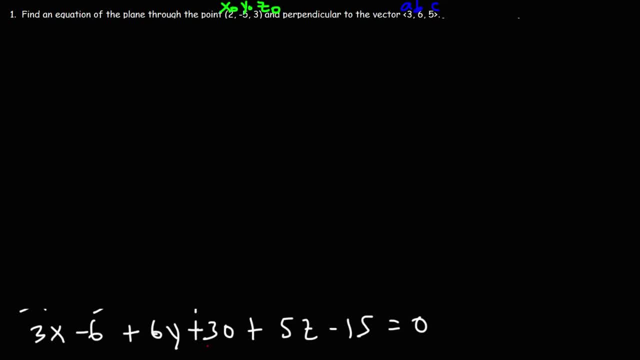 which equals zero. Now the next thing we need to do is we need to combine like terms. So 30 minus 15, that's 15.. 15 plus negative six is nine. So we have three x plus six, y plus five, z and then plus nine. I'm going to take the nine and move it to the other side. 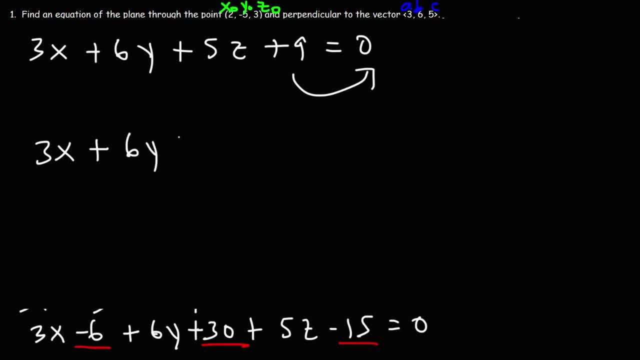 So we have three x plus six y plus five z, and that's equal to negative nine. So this is the equation of the plane that we're going to use to get the equation of the plane. And then we need to the equation of the plane that contains the point 2, negative 5, 3, and it's perpendicular to the. 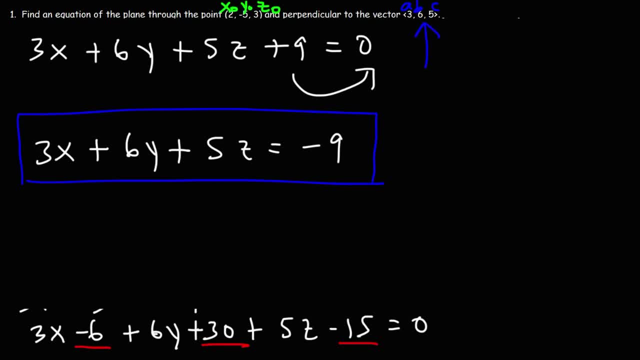 vector 3,, 6,, 5.. So that's how you could find it, But now let's work on another example. For the sake of practice, go ahead and try this problem. By the way, for those of you who are, 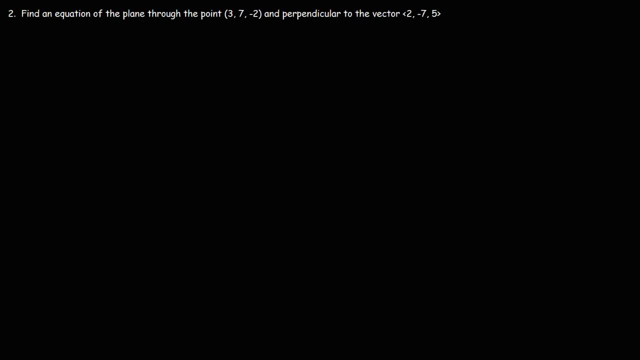 watching this video, and if you haven't subscribed to this channel, feel free to go ahead and do that now, And if you want to receive notification on videos that I'm going to be uploading in the future, don't forget to hit that notification bell. So let's begin. Let's begin by identifying. 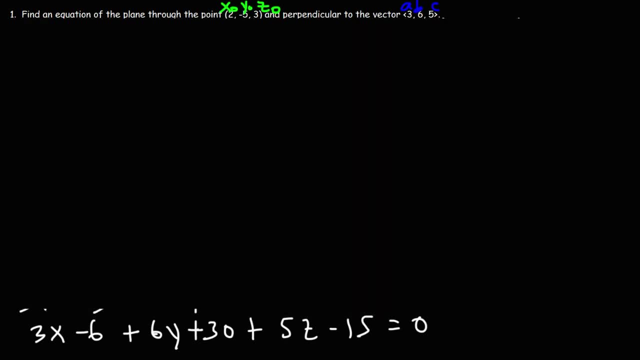 Now the next thing we need to do is we need to combine like terms. So 30 minus 15, that's 15.. 15 plus negative 6 is 9.. So we have 3x plus 6y plus 5z and then plus 9.. I'm going to take the 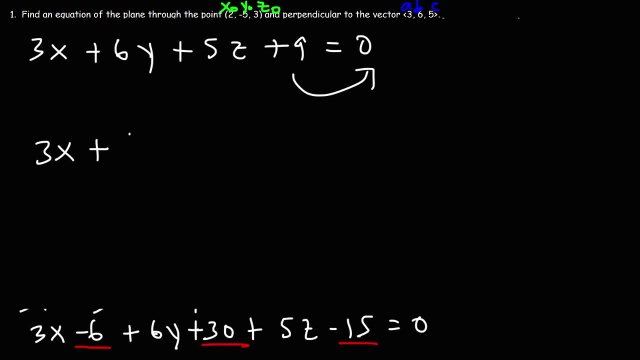 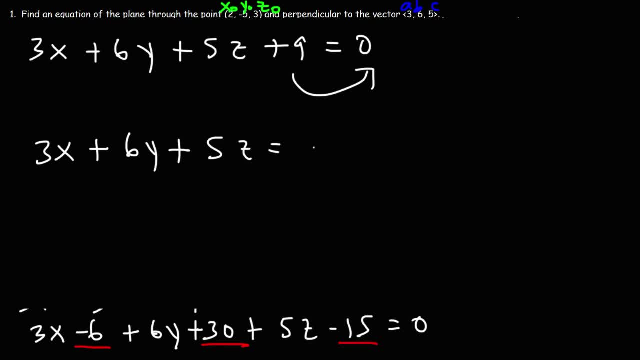 plus 5z, and that's equal to negative 9.. So this is the equation of the plane that contains the point 2, negative 5, 3, and it's perpendicular to the vector 3,, 6,, 5.. So that's how you could. 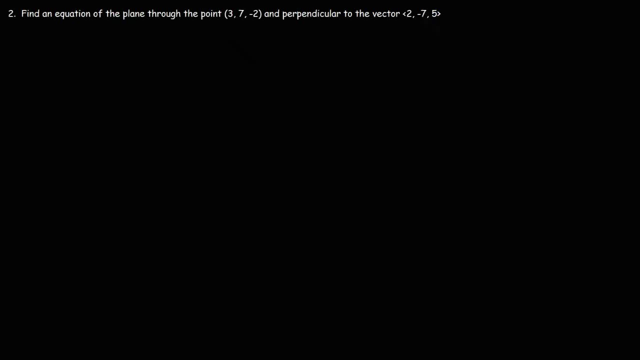 find it, But now let's work on another example. For the sake of practice, go ahead and try this problem. By the way, for those of you who are watching this video, and if you haven't subscribed to this channel yet, please do so. And if you haven't subscribed to this channel yet, please. 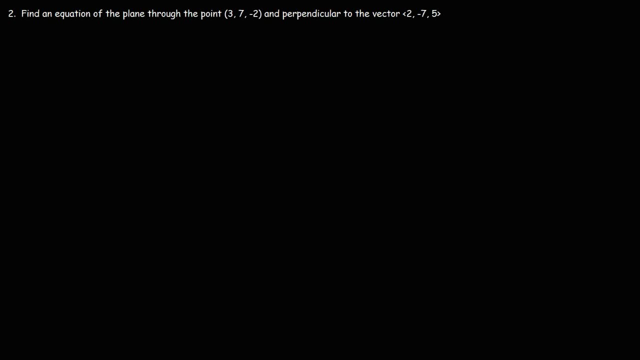 subscribe to this channel. Feel free to go ahead and do that now, And if you want to receive notification on videos that I'm going to be uploading in the future, don't forget to hit that notification bell. So let's begin. Let's begin by identifying the values. So we have our 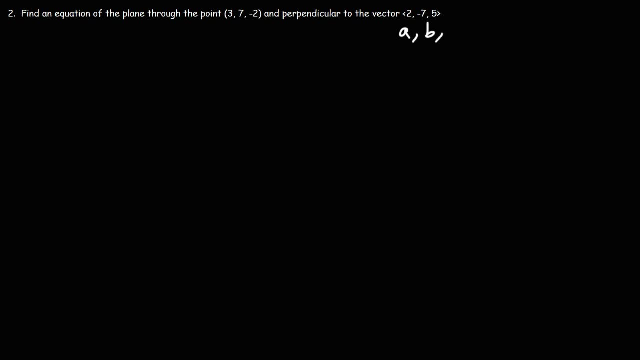 normal vector, which means that a is 2, b is negative, 7, c is 5.. And then we have the point that is on a plane. So x0 is 3, y0 is 7.. z0 is negative 2.. So let's write the formula that we're going to use. So it's a times x minus x0,. 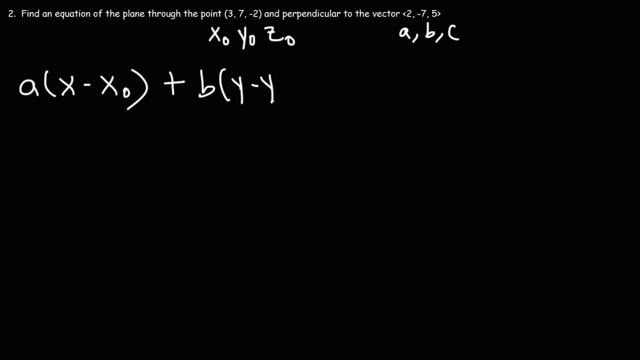 and then plus b times y minus y0,, plus c times z minus z0.. Now all we need to do is plug in the values that we have. So a is 2, x0 is 3, b is negative 7, y0 is 7, c is 5, z0 is negative 2.. So this becomes z plus 2..